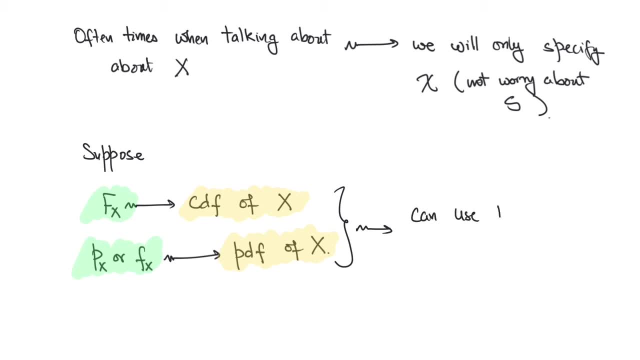 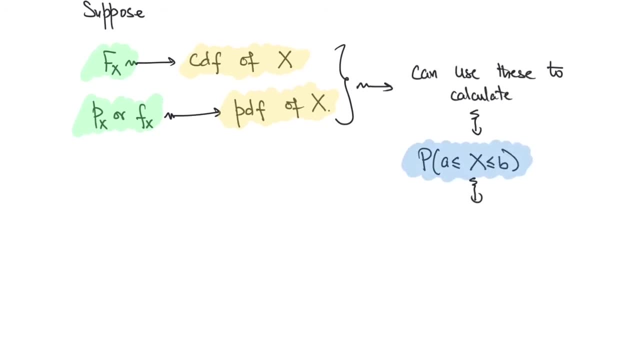 PDF or the PMFs of x. we can use these to calculate the probability that x lies between a and b. That is, the probability that x takes values in the interval a comma b. x is said to be a discrete random variable. if the CDF, the cumulative 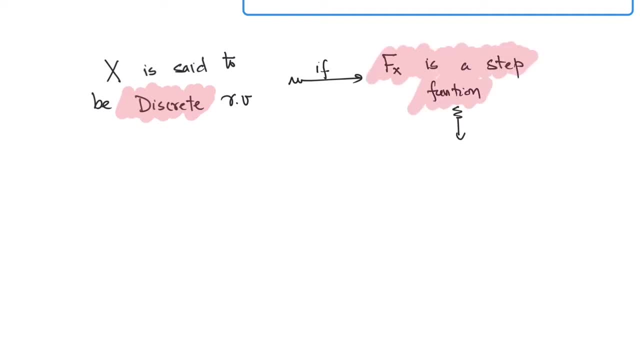 distribution function of x is a step function, In this case script x. the set of values of x will be a discrete subset of r, That is to say that a script x is either going to be a finite set or a countably infinite set. 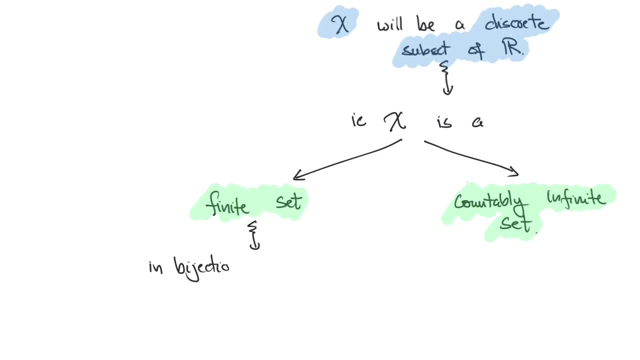 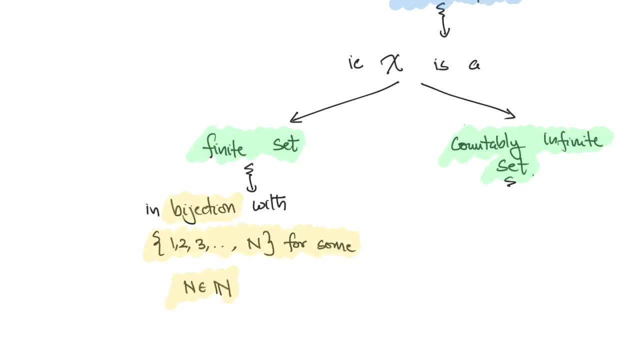 In the case of finite sets, it means that it's going to be in bijection with 1,, 2, 3, up to capital N for some fixed capital N, inside the set of natural numbers N. On the other hand, countably infinite sets are sets that are in bijection with the set of natural numbers. 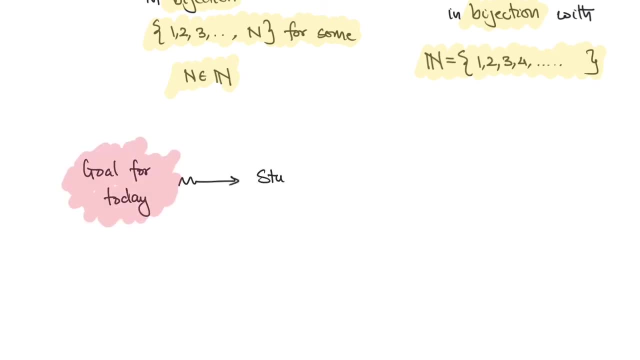 The goal for today is going to be to study random variables which have a finite set for its set of values, That is, we want to calculate the PMF, P sub x, the expected values and the variances of such random variables. The first random variable would be the uniform discrete random variable. We will fix a capital. 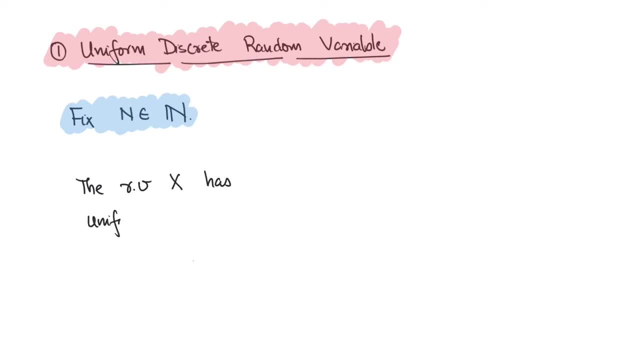 N inside the set of natural numbers, Then the random variable x has a uniform discrete distribution with parameter capital n, if the set of values, script x of this random variable is the set one, two, three up to n. furthermore, for any x inside script x, p, sub x of x is going to be equal to 1 over n, uniformly. 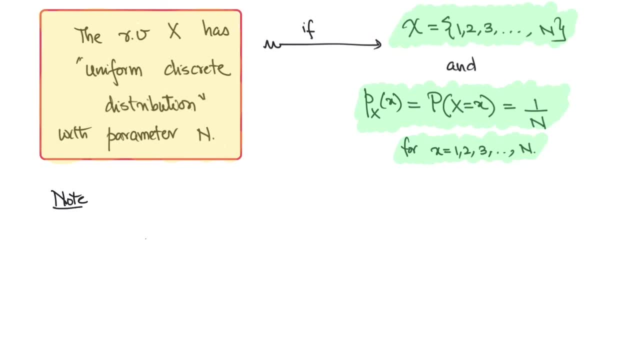 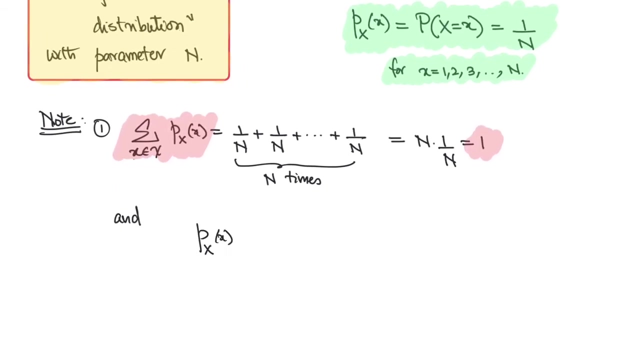 note that if we take the sum over all values of x inside script, x of p sub x of x, you get n times 1 over n, which is equal to 1. also, p sub x of x equals 1 over n, which is a positive number for. 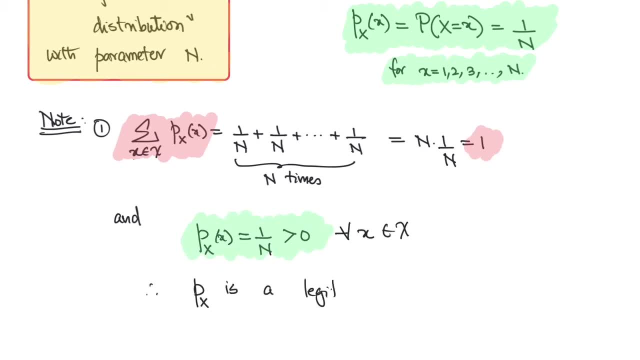 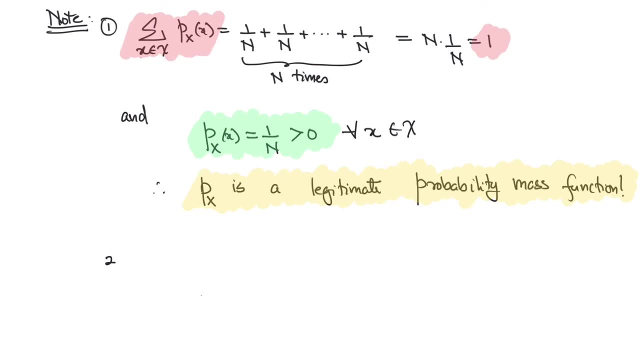 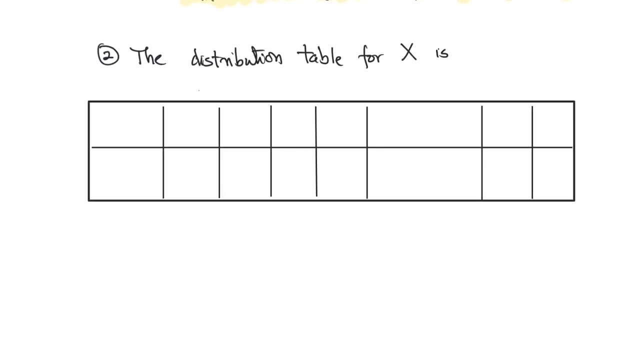 all values of x. so this tells us that p sub x is a legitimate probability mass function. the distribution table for x is computed as follows: we have the values of x being 1, 2, 3, 4 all the way up to n, and the probability that x equals 6 is uniformly equal to 1 over n. in this setting, the expected value of x. 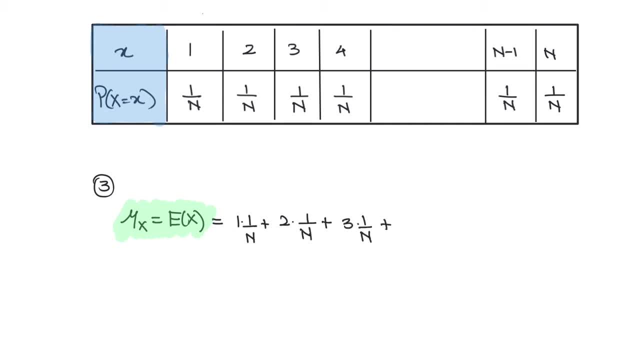 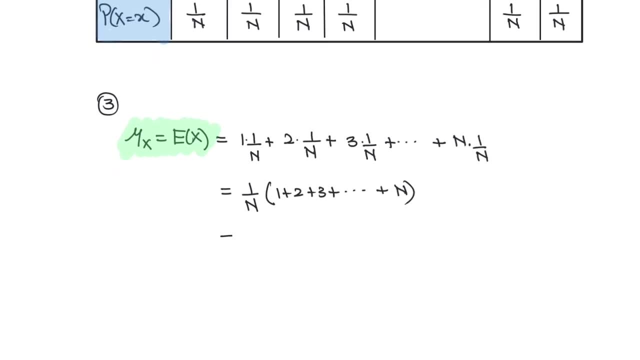 is calculated using the formula for expectation, and in the process we use the formula for the sum of the first n numbers, which is going to be n times n plus 1 divided by 2.. And then we divide out by n. we will get the expected value. 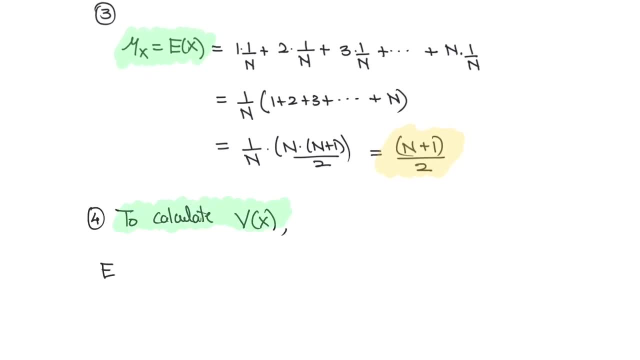 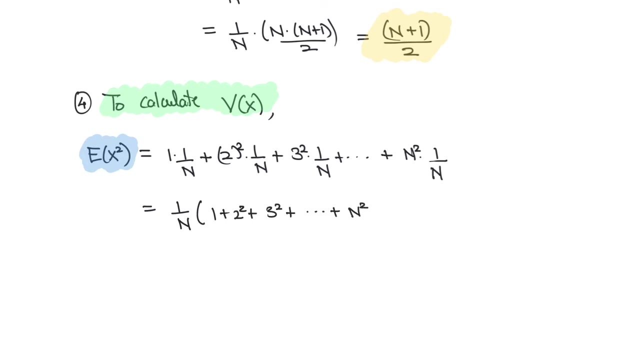 which is going to be n plus 1 over 2.. To calculate the variance, we're going to use the property that the variance of x is the expected value of x squared minus the expected value of x squared. Working through this, we notice that the expected value of x squared 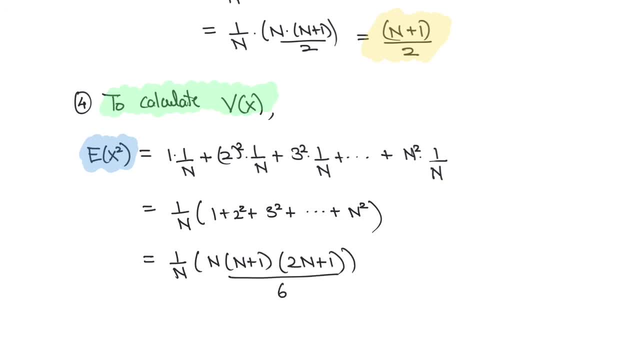 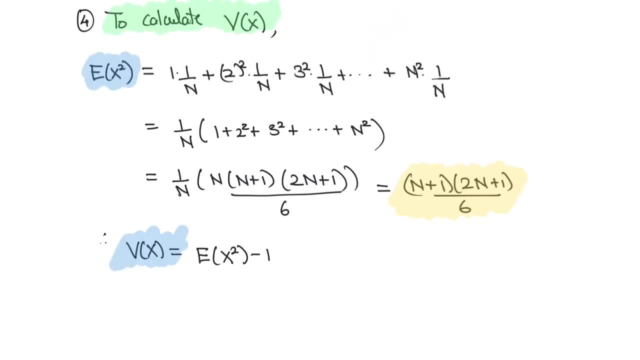 is going to be n plus 1 times 2n plus 1 divided by 6.. And plugging this into the formula for variance, that is, expected value of x squared minus expected value of x, the whole squared, we notice that the variance becomes: 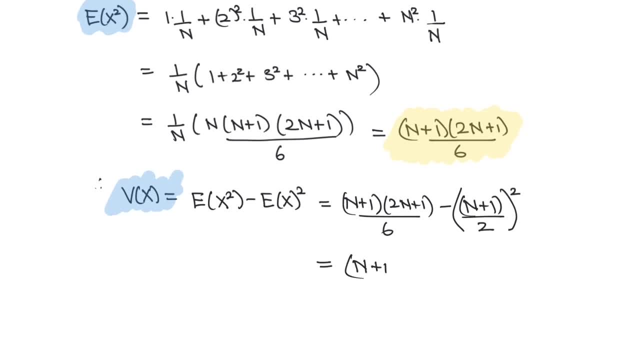 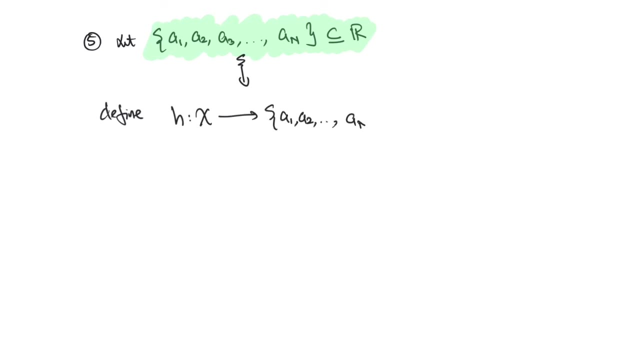 equal to n plus 1 times n minus 1 divided by 12.. We also note that if a1, a2, a3, up to a n is a subset of real numbers, we can define a function h from script x to a1 through a n, where i goes to a i. 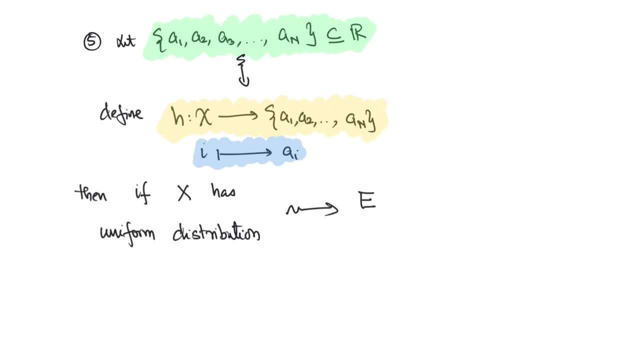 Now, if x has the uniform distribution, then the expected value of h of x is going to be equal to a1 plus a2, all the way up to a n divided by n, which is exactly the mean of these n numbers, And the variance of hx is going to be the variance of these. 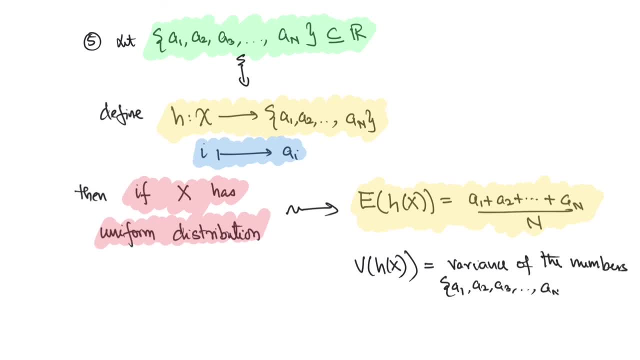 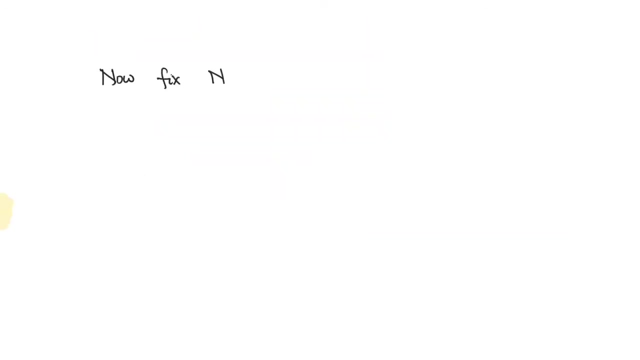 n numbers. In this setting we get that the uniform discrete distribution just gives us the regular mean and the variance of a set of n numbers coming from the set of real numbers. Now fix capital N, capital M and small n to be natural numbers. 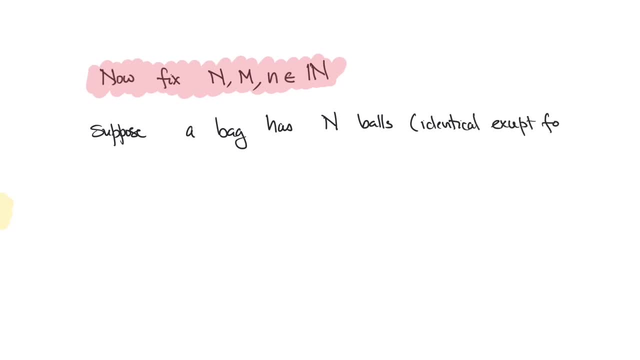 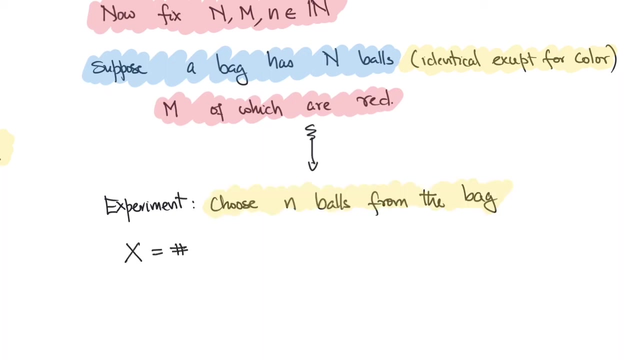 And suppose a bag has capital N balls identical in all respects except for color, and m of these balls are red in color. An experiment consists of choosing n balls from this bag And if we set the random variable x to count the number of red balls, 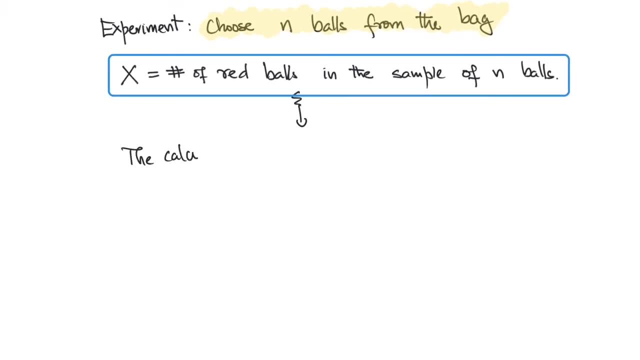 in a sample of small n balls. we want to be interested in calculating the probability mass function of this random variable. However, notice that this depends on how we sample, whether we are sampling without replacement or if we are sampling with replacement When we are sampling without replacement. 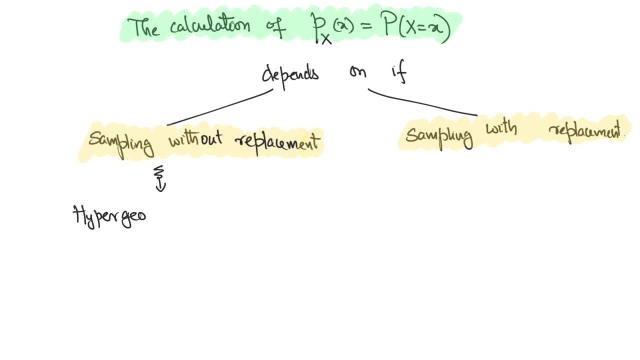 the distribution of this random variable is going to be what is known as the hypergeometric distribution, with parameters capital N, capital M and small n. When we are sampling with replacement, we are going to get the binomial distribution with parameters small n and p. 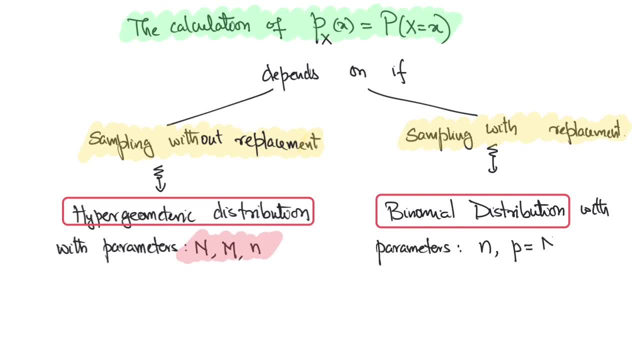 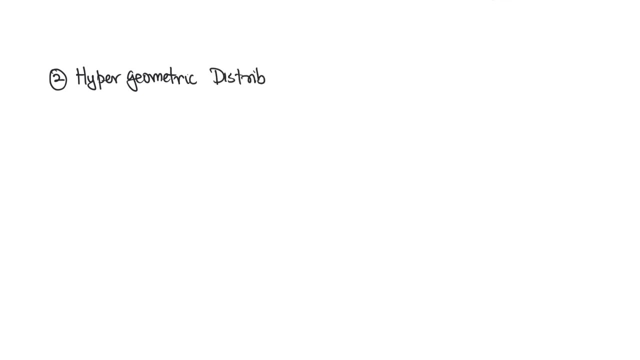 which is going to be equal to capital M over capital N. There is a typo in the video. it should have been: p equals capital M over capital N. We now talk about the hypergeometric distribution. The random variable x is said to have the hypergeometric distribution. 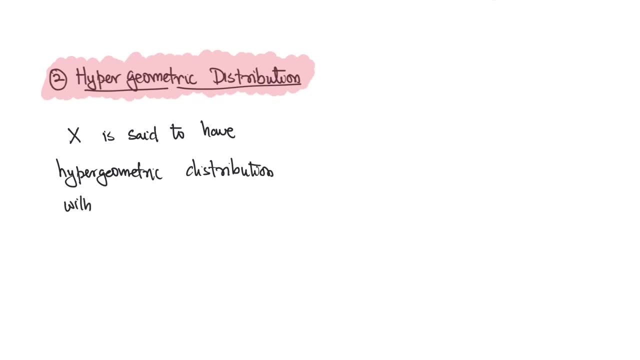 with parameters capital N, capital M and small n. if the random variable takes values in the set 0,, 1,, 2,, 3, up to n and the probability mass function is defined as follows: P of x equals x in this case. 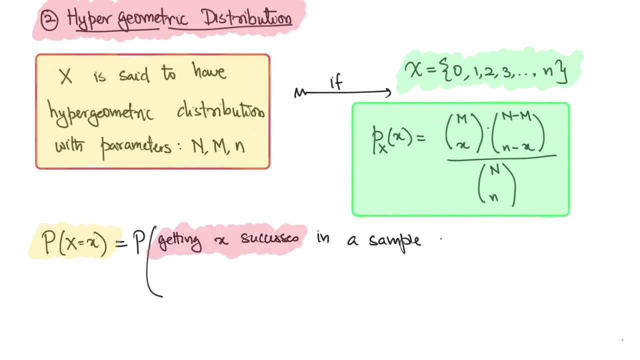 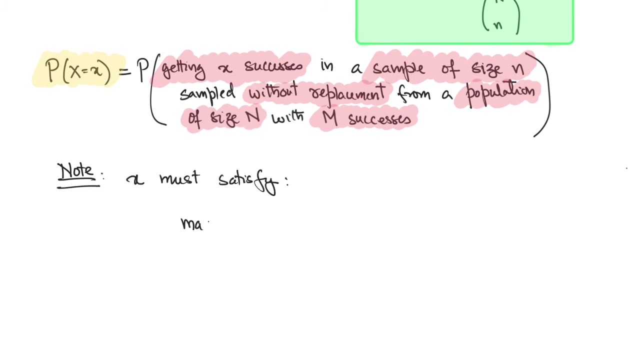 gives us the probability of getting x successes in a sample of size n, sampled without replacement from a population of size capital N with M successes. Note that implicit in this discussion is that capital M has to be less than capital N and that x must lie between the maximum of 0,. 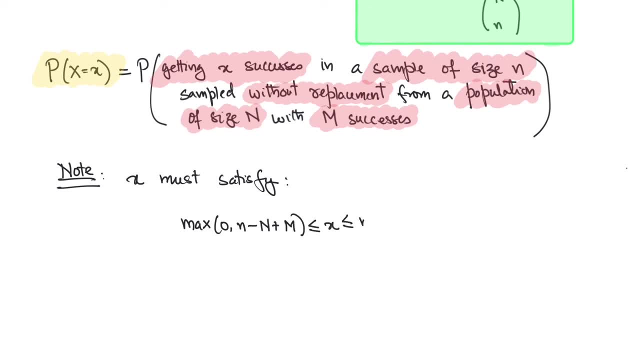 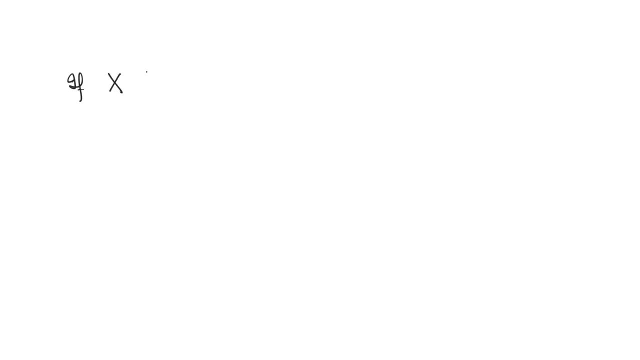 and small n minus capital N plus m and the minimum of small n capital M. We now note the expected value and the variance for the hypergeometric random variable. If x has the hypergeometric distribution with parameters capital N, capital M and small n, then the 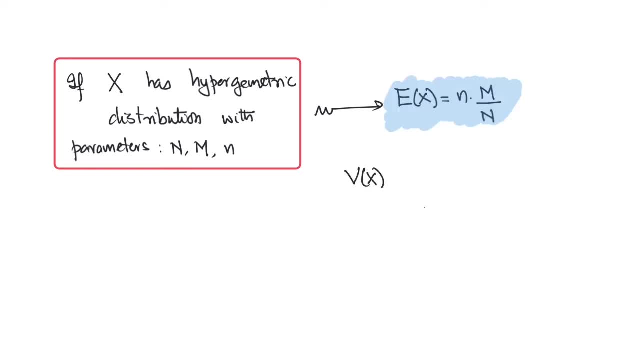 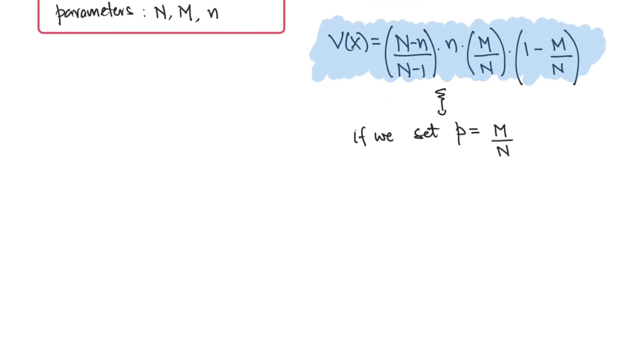 expected value is going to be equal to N times M over capital N and the variance is going to have the following formula: in terms of capital N, capital M and small n. Note that if we set P equals capital M over capital N, the expected value of X is going to be N times P and the 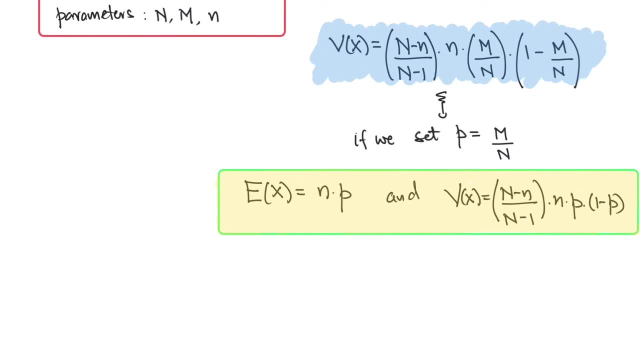 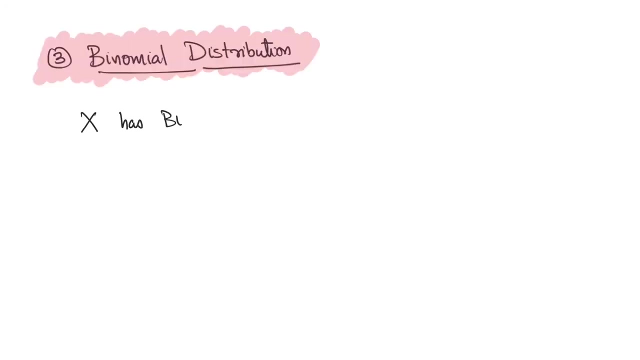 variance of X is going to be N minus small n divided by capital: N minus 1 times N times P times 1 minus P. We next talk about the binomial distribution. We will say that the random variable X has the binomial distribution with parameters small n and small p. 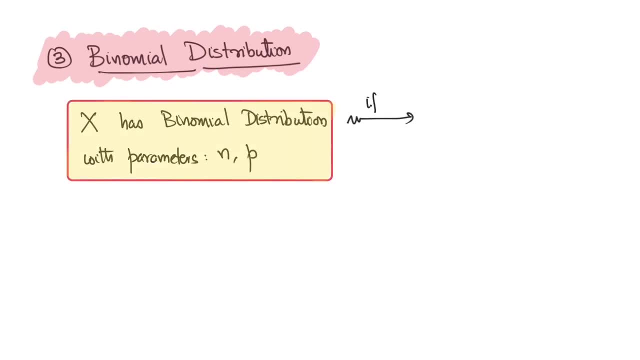 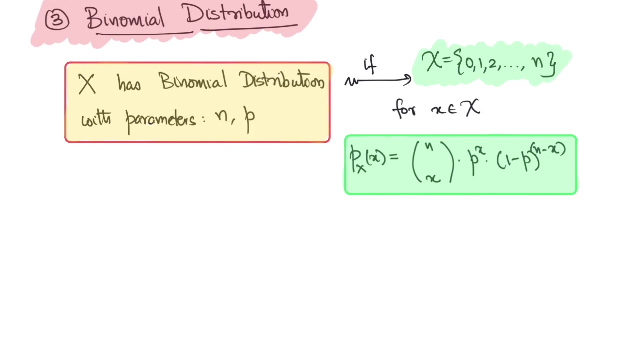 if the set of values equals the set 0,, 1,, 2, up to N and if for any X inside script X, the probability of X equals small, x is going to be equal to N. choose X times P to the X times 1. 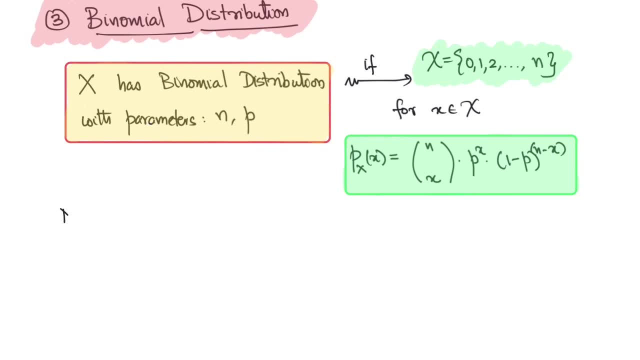 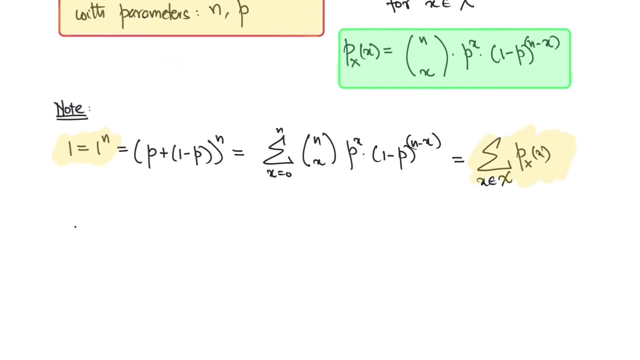 minus P to the N minus X. This is called the binomial distribution, because we use the binomial formula to show that P is equal to N minus P Sub X is in fact a PMF, that is, a probability mass function. When working with the binomial, 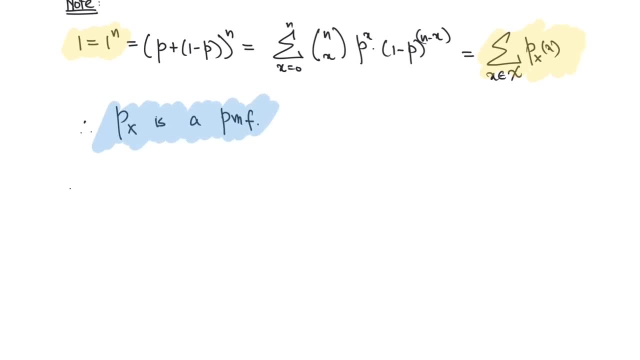 distribution, N is typically going to be the size of a sample and P is going to be the probability of getting a success on every trial. So if X has the binomial distribution with parameters N and P, then the expected value of X is going to be equal to N times. 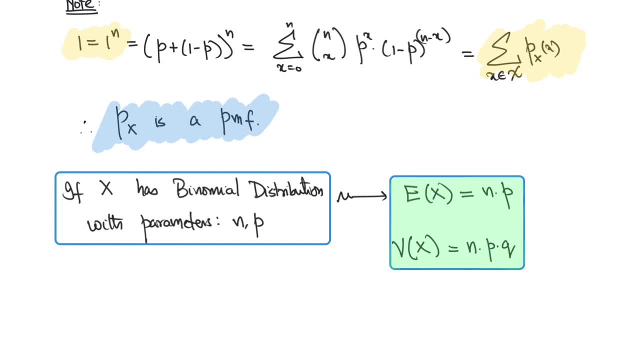 P Sub X is in fact a PMF, that is, a probability mass function. When working with the binomial ungefährques Is going to be equal to N times P times Q, where KY 4002 000 YK Undercolored.